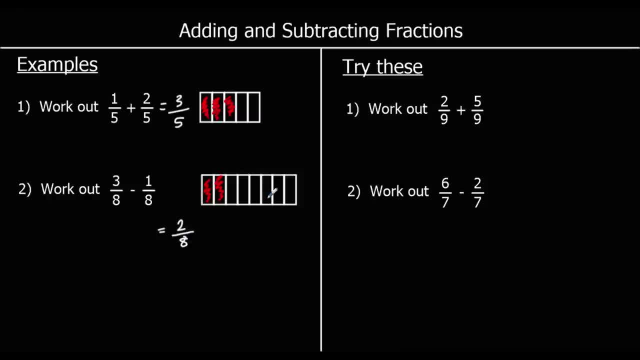 And if we wanted to simplify this answer, two and eight are both even, they're both in the two times table. So we can half the top and the bottom, and say that two-eighths is the same as one-quarter. 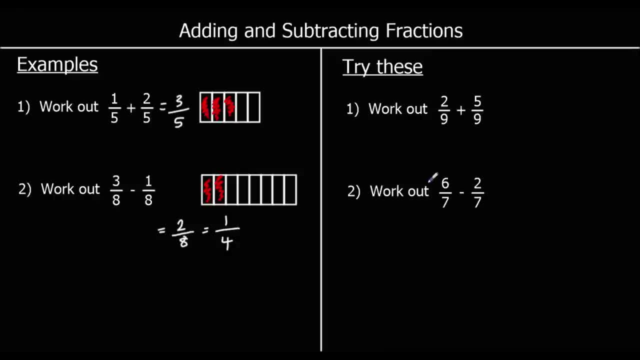 Question one, work out two-ninths plus five-ninths. Two of something plus five of something is seven of something. And they are ninths. So two-ninths plus five-ninths is seven-ninths. 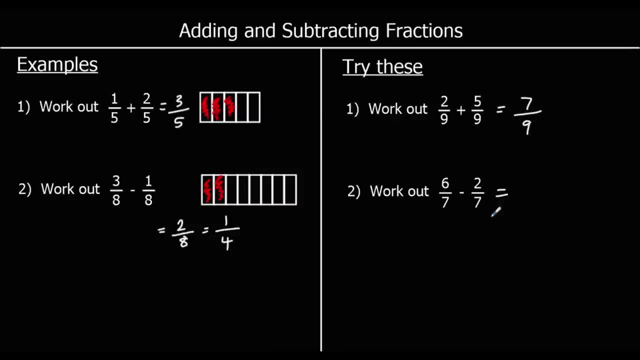 And taking away is the same thing. So six of something, take away two of something, is four of something. So six-sevenths, take away two-sevenths, is four-sevenths. 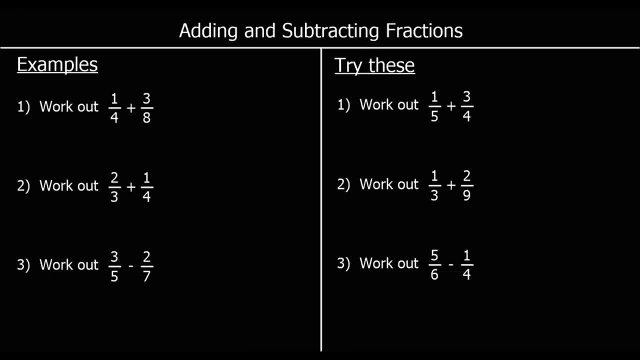 In these questions, we are being asked to add and subtract fractions with different denominators. The way we do that is to change the fractions using equivalent fractions, to make the denominators the same. And then once we've got the denominators the same, we can add or subtract them as before. The first question says one-quarter plus three-eighths. So we're looking to make the denominators the same, which means we're looking for a number in the four-times table and the eight-times table. So what number is in the four-times table and the eight-times table? Well, eight. Eight is in both the times tables. So if we multiply the top and bottom of one-quarter by two, to keep a fraction equivalent, we need to multiply top and bottom by the same thing. 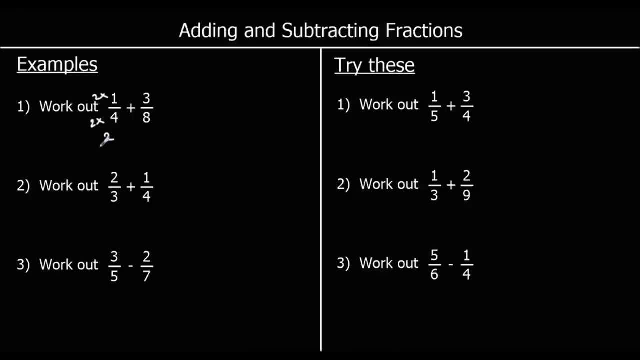 So two times one is two. Two times four is eight. So we're saying one-quarter is the same as two-eighths. 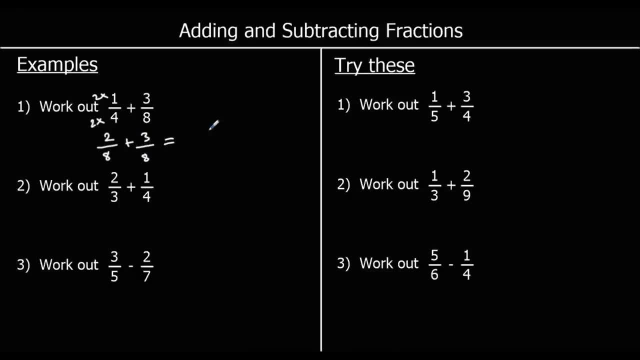 So we can do two-eighths. Plus three-eighths, two of something plus three of something is five of something. So two-eighths plus three-eighths is five-eighths. 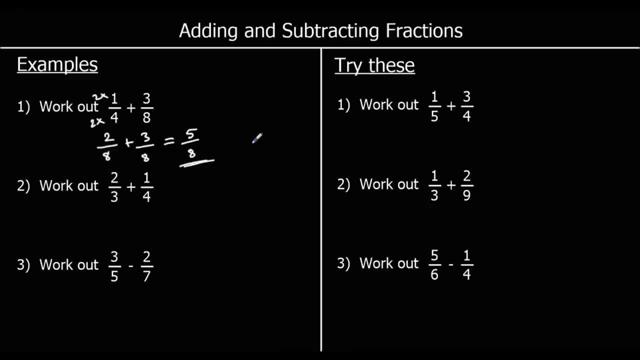 For question two, we're looking for a number in the three-times table and the four-times table. And we can do this this time by doing three times four. So twelve is in both the times tables. Because twelve is three times four. 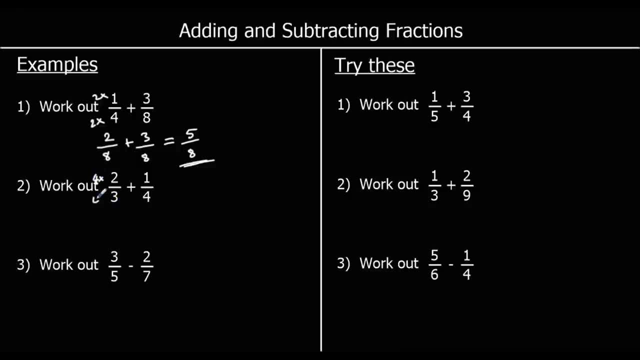 So we can multiply top and bottom of two-thirds by four and the top and bottom of one-quarter by three. 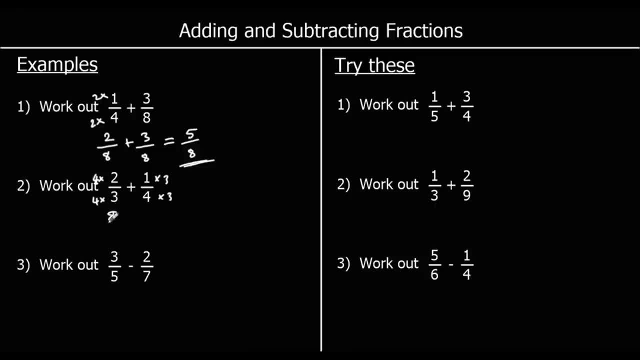 Which will give us eight-twelfths plus three-twelfths. And eight of something plus three of something is eleven of something. So eight-twelfths. 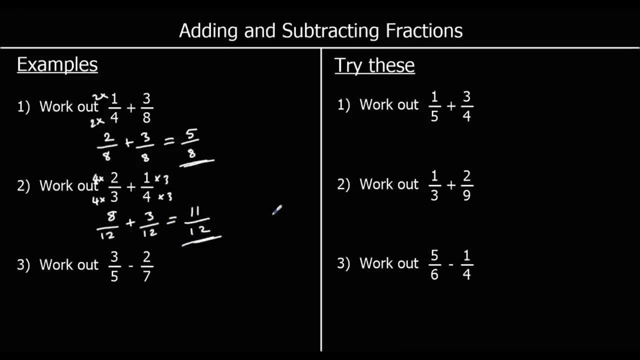 So eight-twelfths plus three-twelfths is eleven-twelfths. 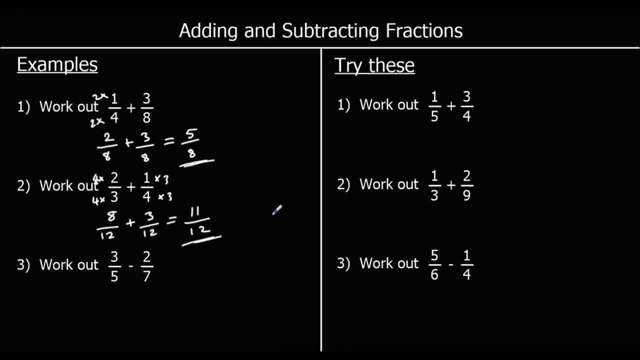 We've got three-fifths take away two-sevenths. But we're going to follow the same steps. We're going to make the denominators the same. 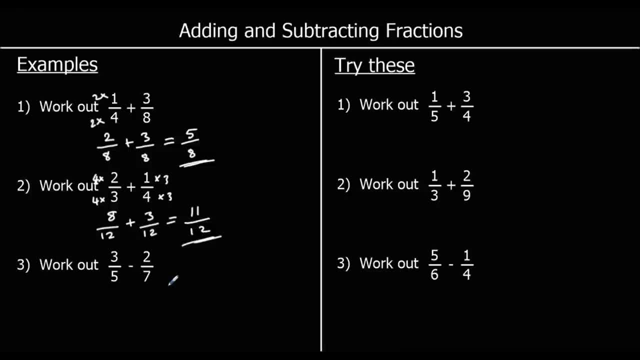 And what number is in the five-times table and the seven-times table? Well, thirty-five is five times seven. 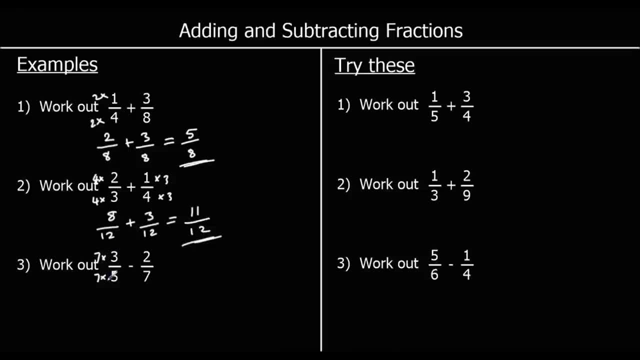 So if we multiply top and bottom of three-fifths, two-fifths by seven and top and bottom of two-sevenths by five we get twenty-one-thirty-fifths minus ten-thirty-fifths. 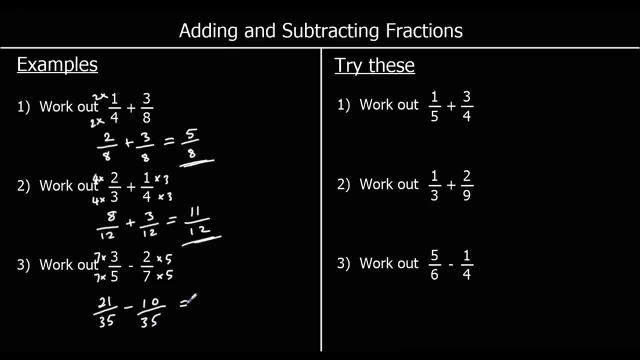 So twenty-one take away ten is eleven. So twenty-one-thirty-fifths take away ten-thirty-fifths is eleven-thirty-fifths. 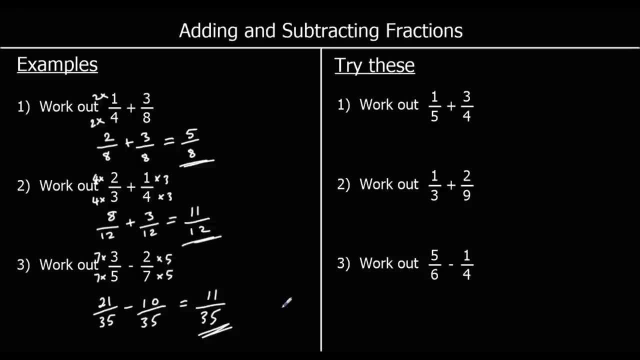 Okay, three for you to try. So give them a go. Here we go. 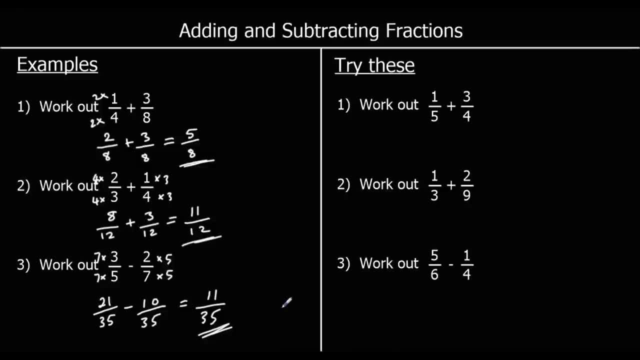 Question one. Work out one-fifth plus three-quarters. 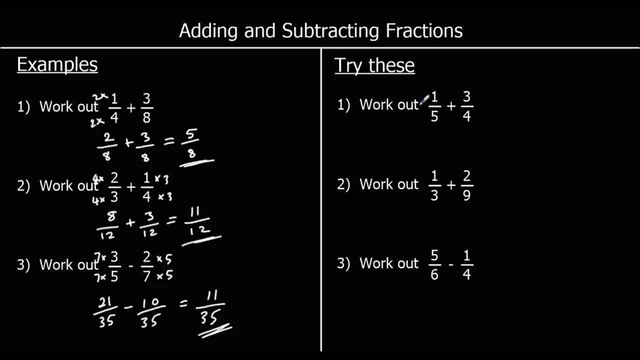 So we need to make the denominators the same. And we're going to do that by multiplying the top and bottom of one-fifth by four. And the top and bottom of three-quarters by five. Which will make both of the denominators twenty. So we've got four-twentieths. Plus fifteen-twentieths. Four plus fifteen is nineteen. So four-twentieths plus fifteen-twentieths is nineteen-twentieths. For question two. We've got thirds and ninths. 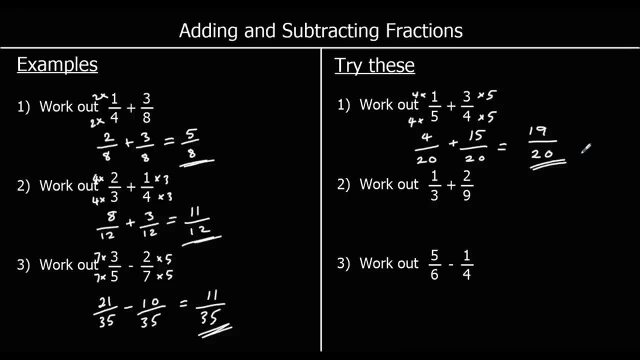 And the smallest number in both the times tables this time is nine. 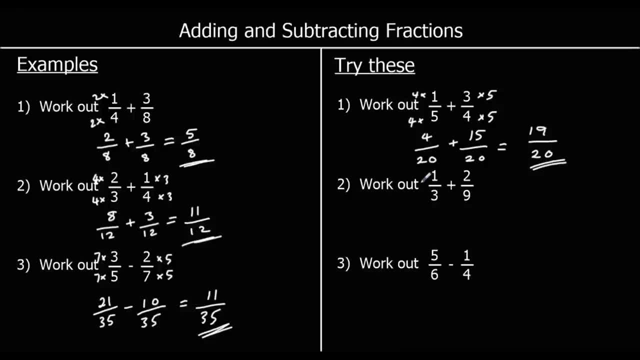 So if you did. You could. Multiply this side one-third top and bottom by nine. 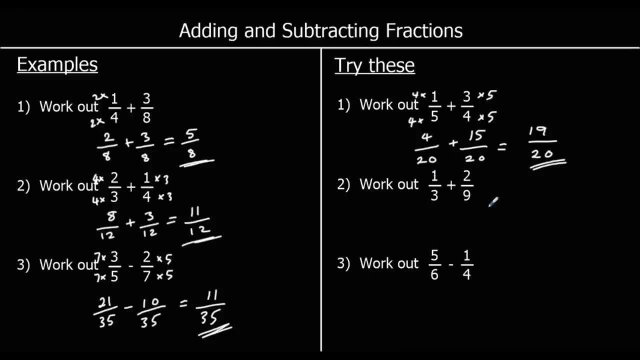 And two-ninth top and bottom by three. And get twenty-seven on the bottom. Then you could simplify the answer at the end. But the easiest way to do it. 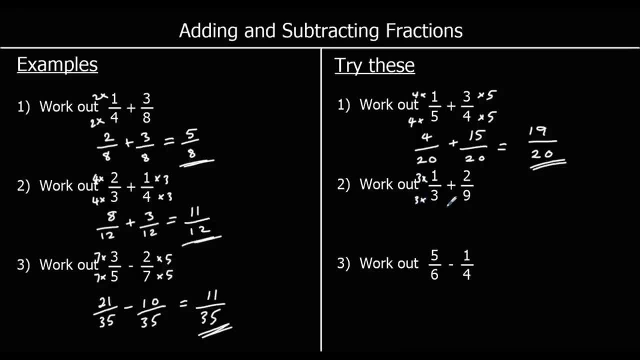 Is to multiply. Top and bottom of one-third by three. Which will give us three-ninth. 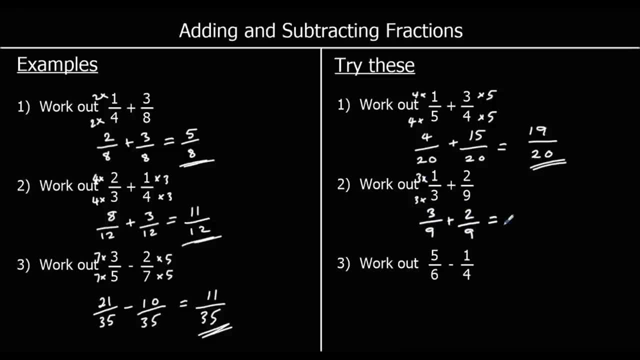 And so we've got three-ninth plus two-ninth. Which is two-ninth. Which is five-ninth. And question three. 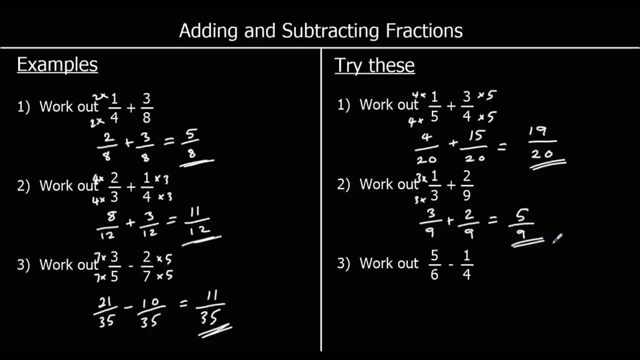 This time the smallest number in the six times table. And the four times table. Is twelve. 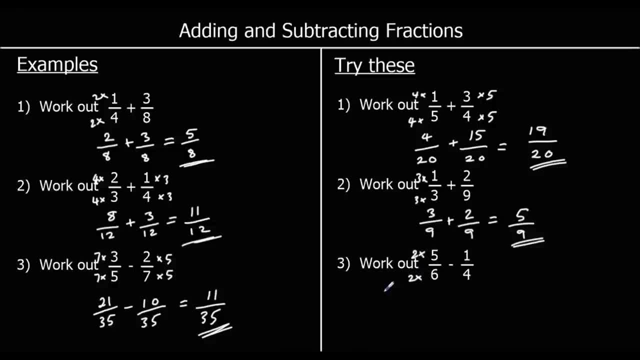 So if we multiply. Five-sixths. 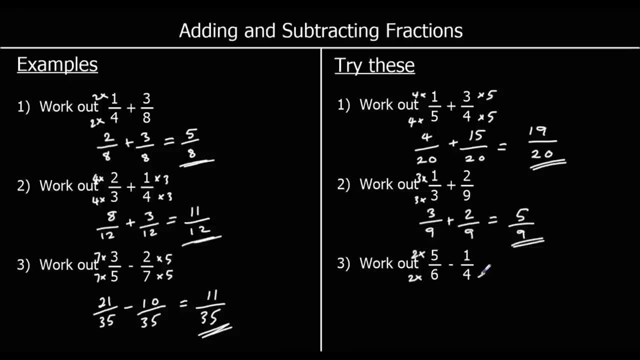 The top and bottom multiplied by two. And one-quarter multiply the top and bottom by three. We get ten-twelfths. 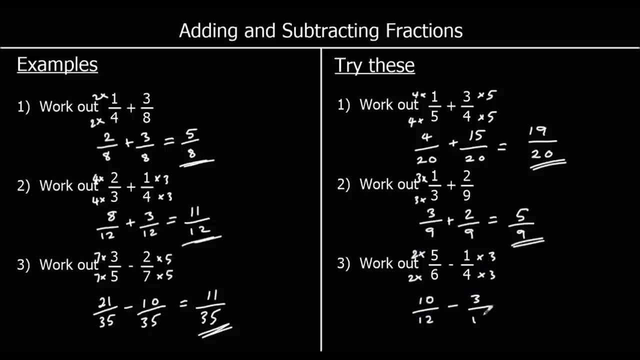 Take away. Three-twelfths. Ten take away three is seven. 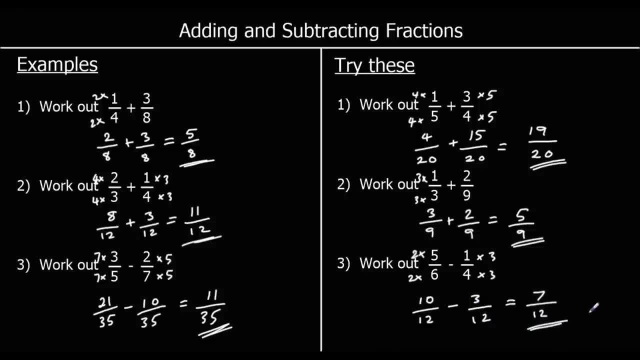 So ten-twelfths take away three-twelfths. Is seven-twelfths. 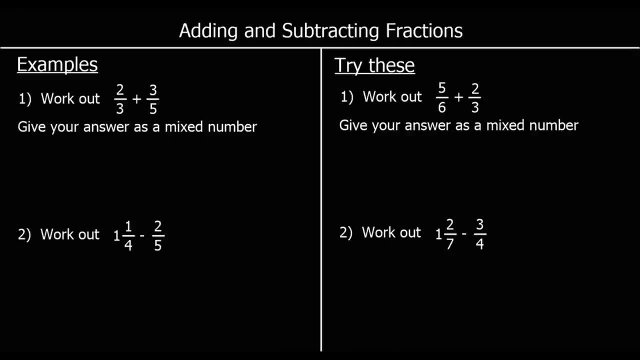 Here we have some more examples. This time we're looking at. Fractions that go over one. 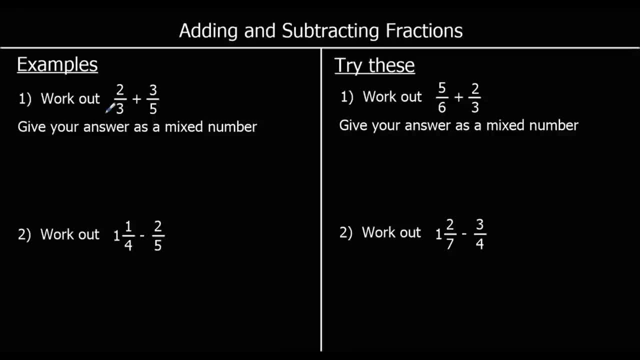 So we've got two-thirds plus three-fifths. We're going to follow the same steps. We need to make the bottom numbers the same before we can add them. So we can make them both fifteen. 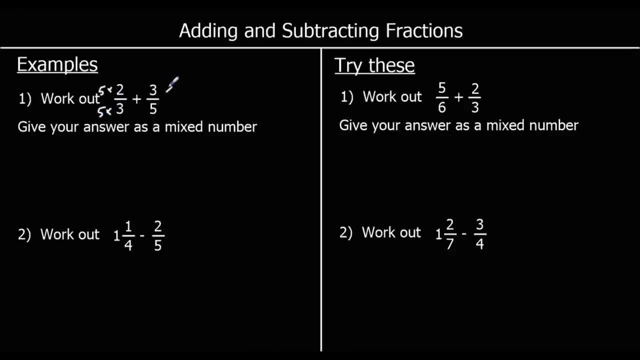 By timesing top and bottom of two-thirds by five. And top and bottom of three-fifths by three. So that will give us ten-fifteenths. Plus nine-fifteenths. So ten of something plus nine of something. Is nineteen. So that means we've got nineteen-fifteenths. 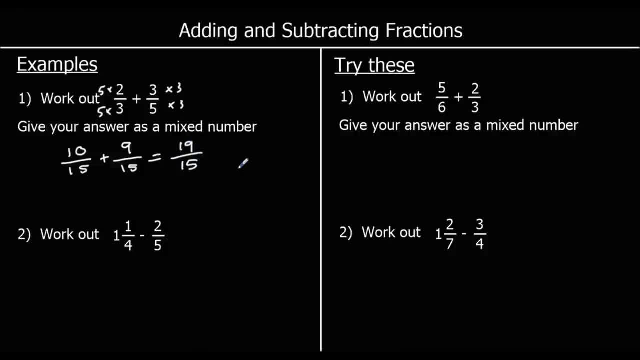 And we can see that this goes over one whole. So fifteen-fifteenths. 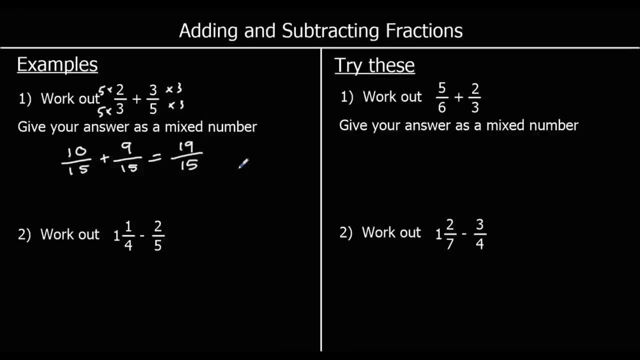 Is a whole. If I've got fifteen-fifteenths. I can say that's one. 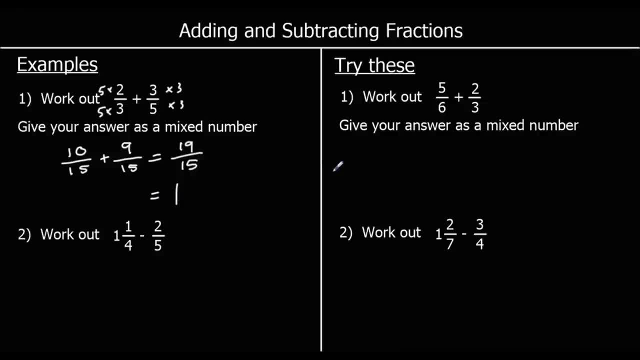 One whole one. How many more fifteenths do I have? 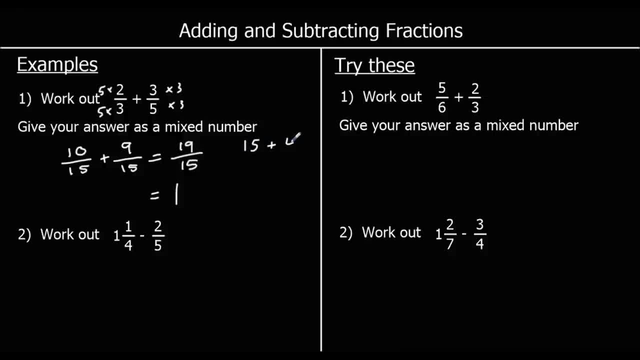 So we've got fifteen. Plus four to make. Nineteen. So we can say it's fifteen-fifteenths. 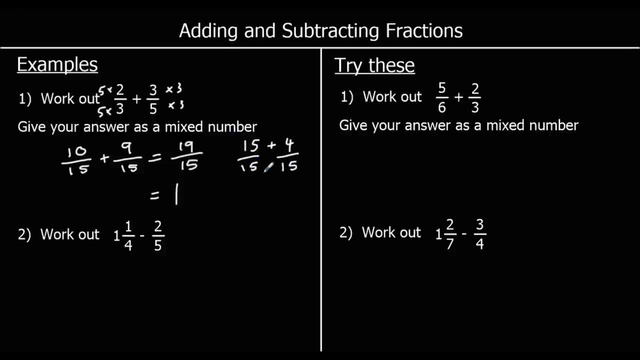 And four-fifteenths. Or one whole one. And four-fifteenths. 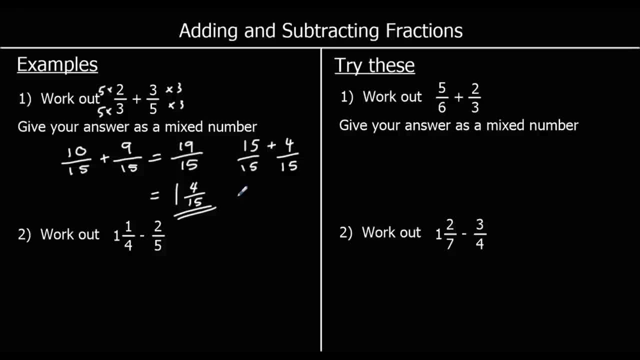 So we can say the answer is one whole one. And four-fifteenths. 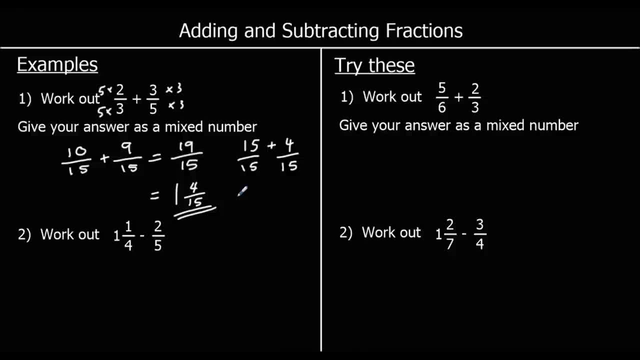 For question two. We've got one. And one-quarter. Take away two-fifths. 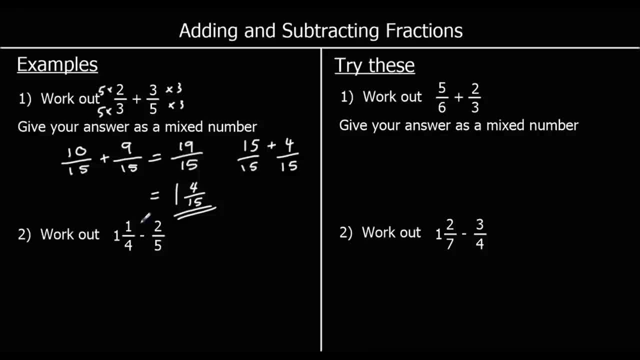 So. We're going to change. The mixed number. Back into a top heavy fraction. So one whole one. In quarters. Is four-quarters. So four-quarters. And one-quarter. Is five-quarters. 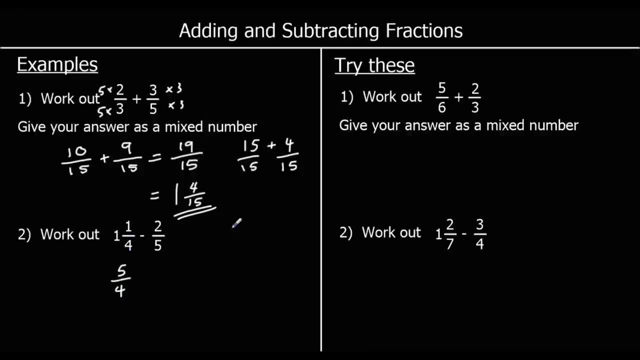 So we can say that one whole one. And one-quarter. So a whole. Circle. In quarters. Plus. Another quarter. Means we've got five-quarters. 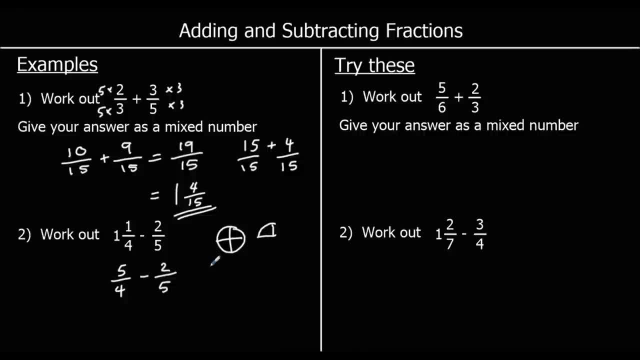 And we're taking away two-fifths. So to take these away. We're going to make the denominators the same first. So if we multiply. Top and bottom by five. And top and bottom by four. We can make both the denominators twenty. So five-fives are twenty-five. Five-fours are twenty. So twenty-five-twentieths. 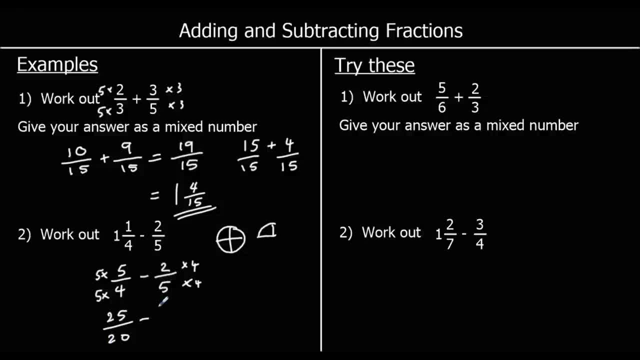 Take away. Two-fours are eight. Five-fours are twenty. 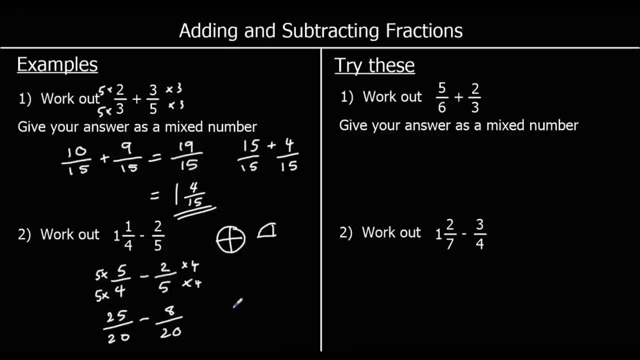 So twenty-five-twentieths. Take away eight-twentieths. Twenty-five take away eight. Is. Seventeen. 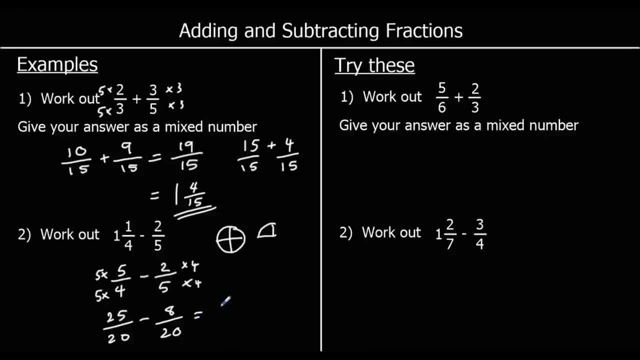 So we've got. Seventeen-twentieths. And. Five-fives. Okay. Two for you to try. So give these ones a go. 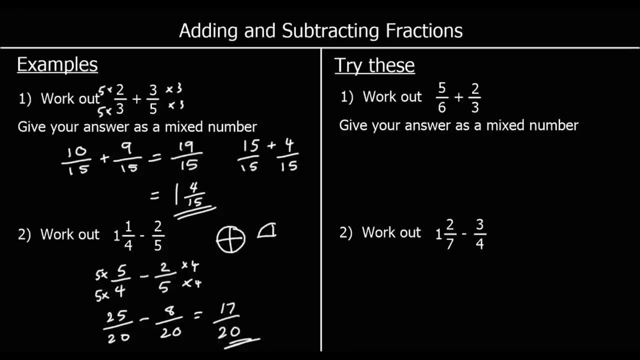 Question one. Work out five-sixths. Plus two-thirds. 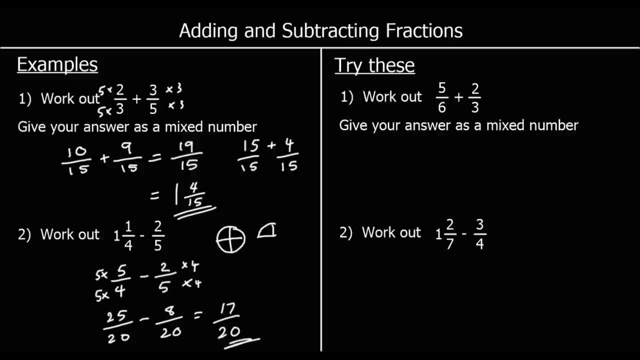 So to add them. We need to make the bottom numbers the same. The denominators the same. And. Easiest way of doing that. Is to make them both out of six. So. Double top and bottom of two-thirds. 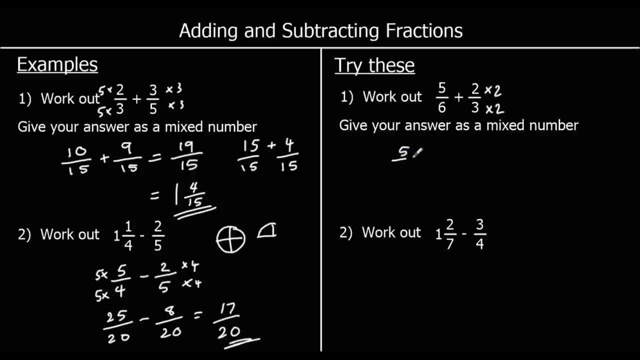 We're going to have. Five-sixths. Plus. Four-sixths. 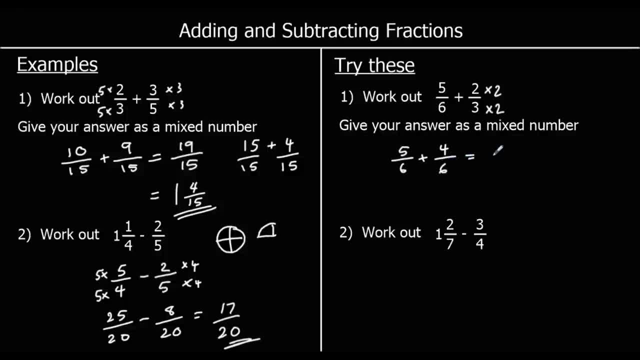 And five plus four. Is nine. So that makes nine-sixths. And we can. Simplify that. Nine and six are both in the three times table. 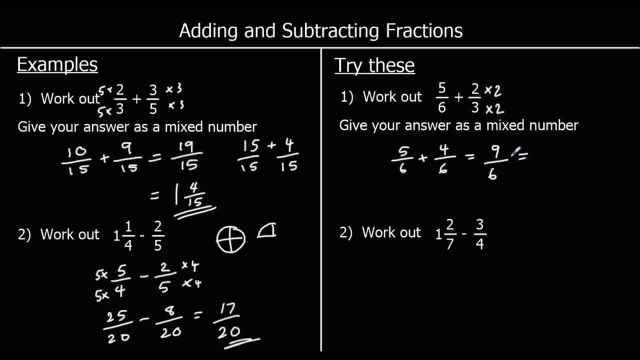 So. Nine is three-threes. Six is. 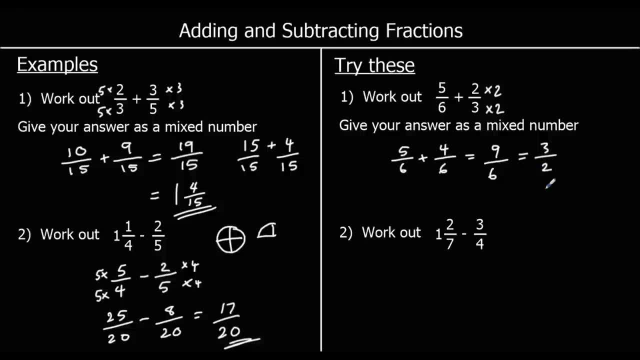 Two threes. So we've got three over two. We need to give our answers a mixed number. We've got a top heavy fraction at the moment. Three is bigger than two. So it's bigger than one. So we can say that. 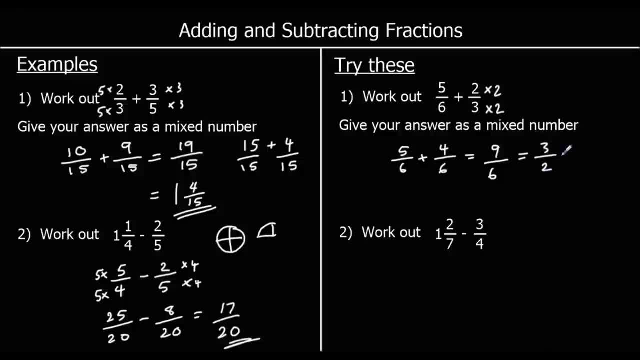 Two. Halfs. Make a whole. So we've got two halves. Plus another half. To make three halves. So we've got one whole one. And one half. Question two. 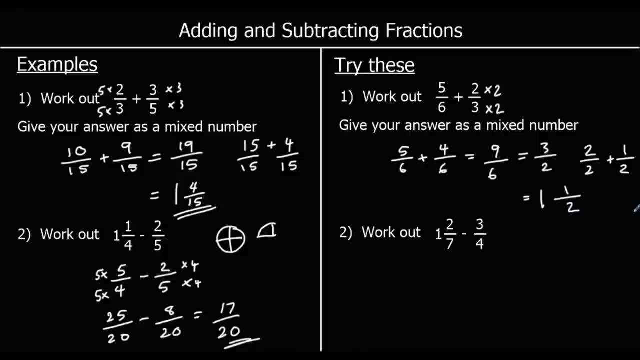 Work out. One and two-sevenths. Take away three-quarters. 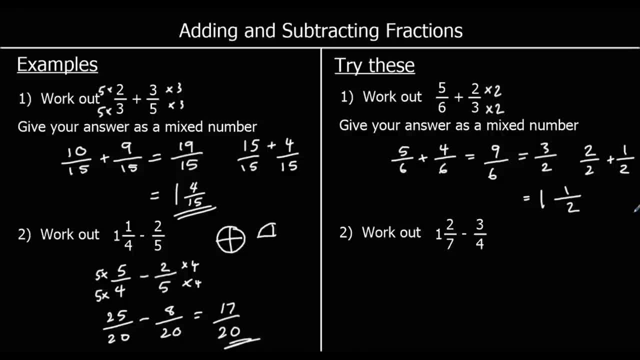 So. We're going to change the mixed number. Back to a top heavy fraction. So one. 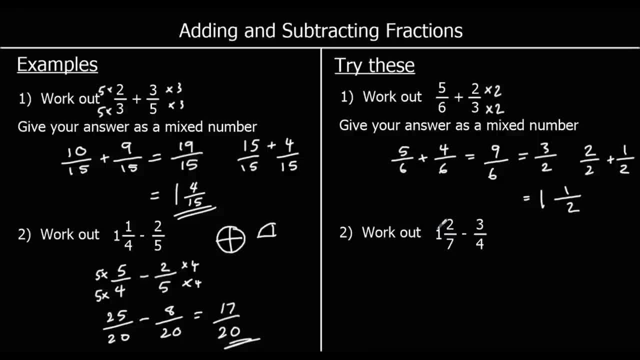 Whole one. Is seven-sevenths. So a whole one is seven-sevenths. 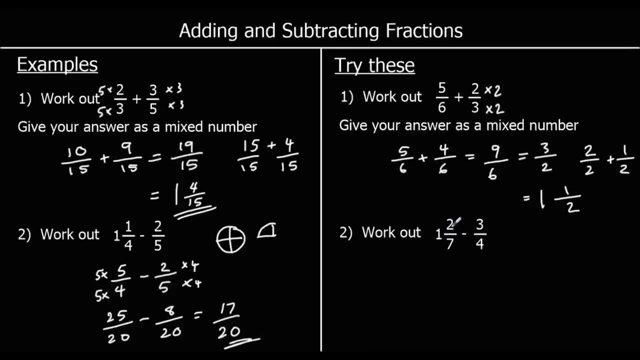 And we've got. Seven-sevenths and two-sevenths. Seven and two make nine. So that's nine. Sevenths. So a whole one. 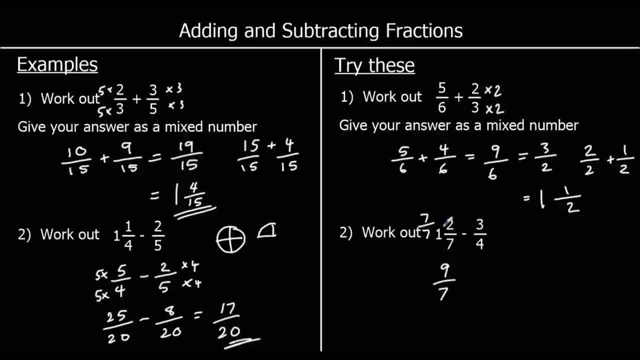 This whole one. Means seven-sevenths. So seven-sevenths and two-sevenths. Is nine-sevenths. 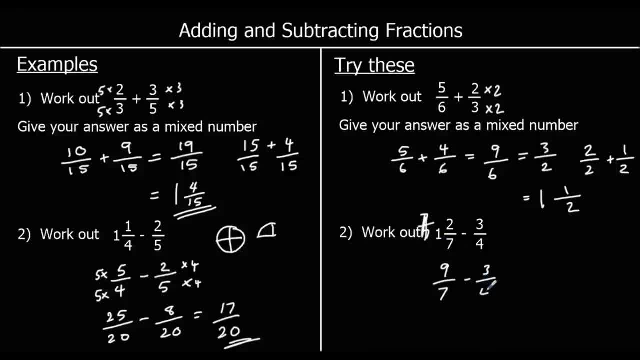 So we've got nine-sevenths. Take away three-quarters. To take them away. We need to make the bottom numbers the same. And. 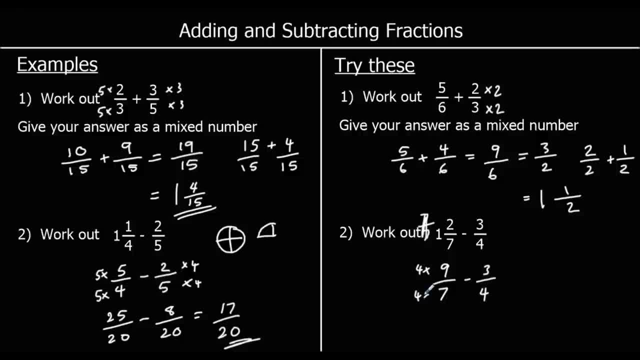 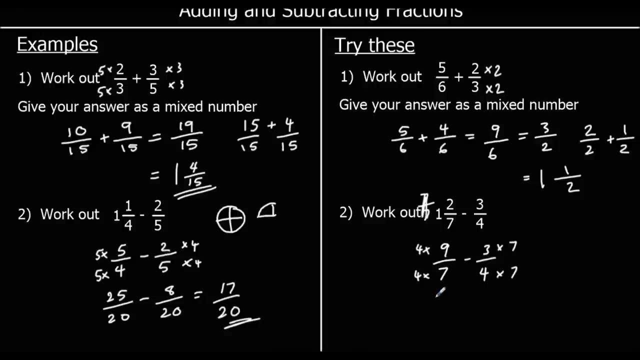 We can do that by multiplying. Top and bottom. Of nine-sevenths by four. And top and bottom of three-quarters. By seven. And then both the bottom numbers. Will be twenty-eight. So we have. Four-nines. 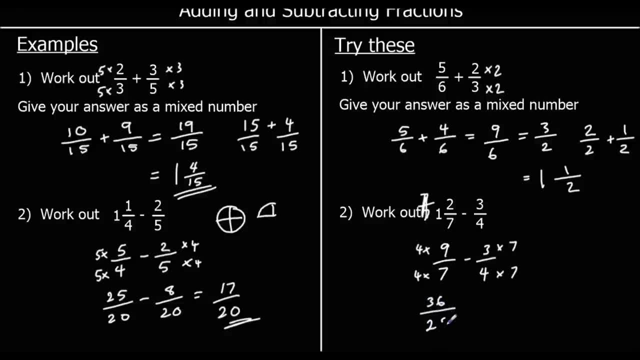 Which is thirty-six. Over four-sevenths. Which is twenty-eight. Take away three-sevenths. Which is twenty-one. Over twenty-eight. So thirty-six. Take away twenty-one. Is fifteen. 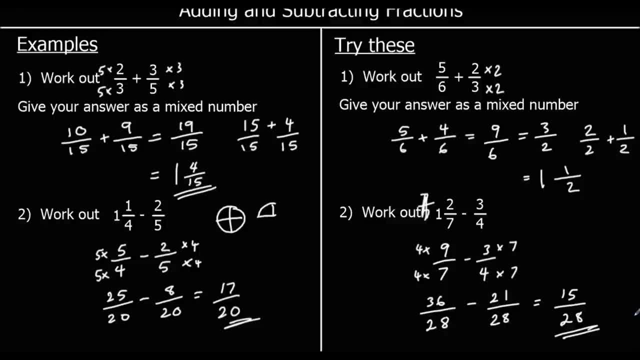 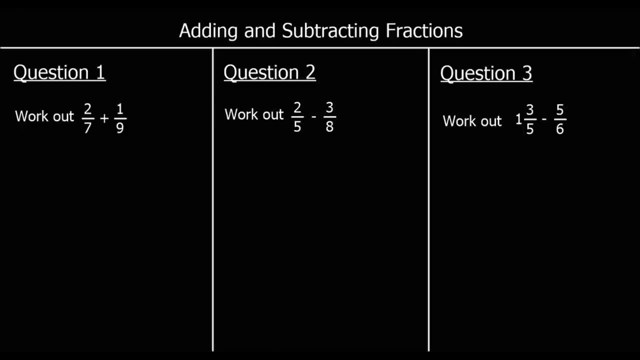 Twenty-eight. To finish up. We've got three questions here. So pause the video. Give them a go. And press play when you're ready for the answers. 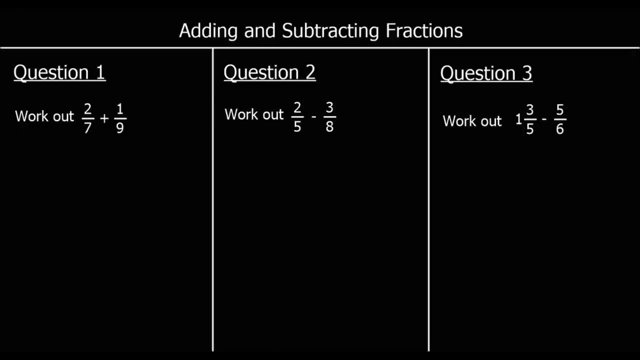 Question one. Two-sevenths. Plus one-ninth. 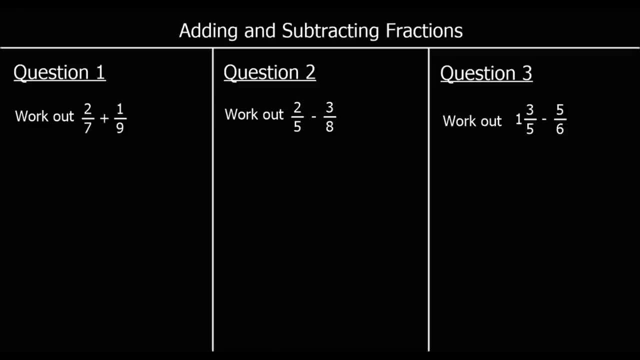 We need to make the denominators the same. And. We'll do that by multiplying. Top and bottom of two-sevenths by nine. And top and bottom of one-ninth. By seven. And both the denominators will be the same. Because nine times seven. Is the same as. 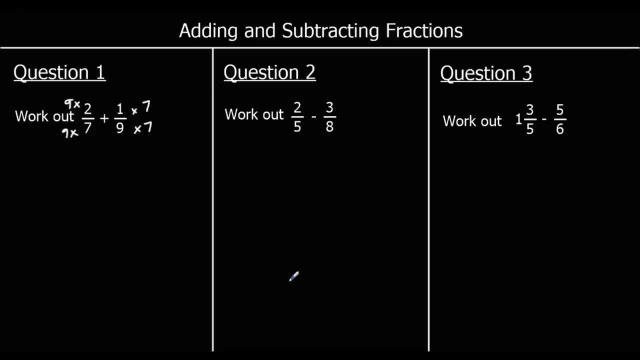 Well nine times seven. They're both sixty-three. So we have. Nine times two. Which is eighteen. Over sixty-three. Plus. Seven over sixty-three. And eighteen. 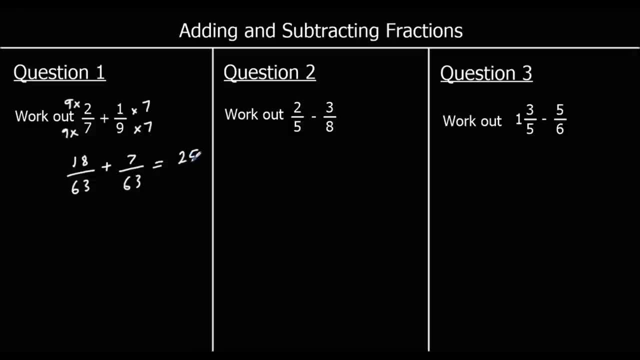 Plus seven is twenty-five. So we've got twenty-five. Over sixty-three. 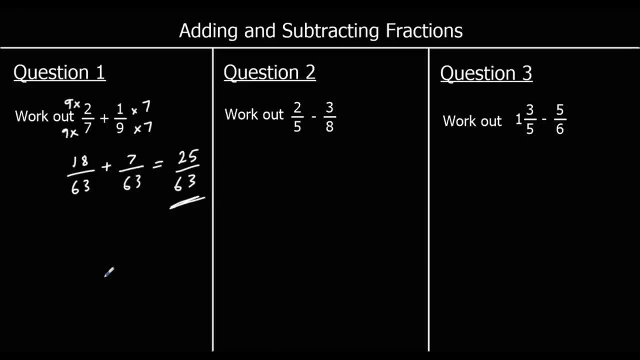 Question two. We're going to multiply. Top and bottom. Of two-fifths by eight. Top and bottom of three-eighths by five. So. 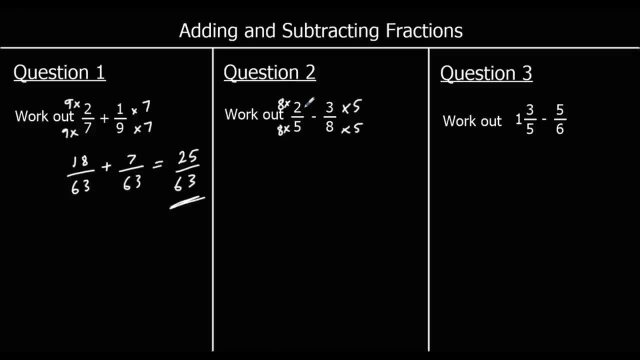 They'll both be out of forty. So two. Eighths of sixteen. Over forty. Minus. Three-fifths. Which is fifteen. Over forty. Sixteen minus fifteen. Is one. 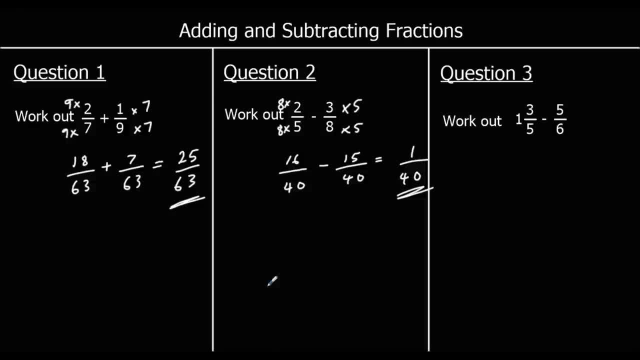 So we've got one-fortieth. And for question three. We're going to change. The fraction. Into top-heavy first. Change the mixed number. Into top-heavy. So we've got one whole one.